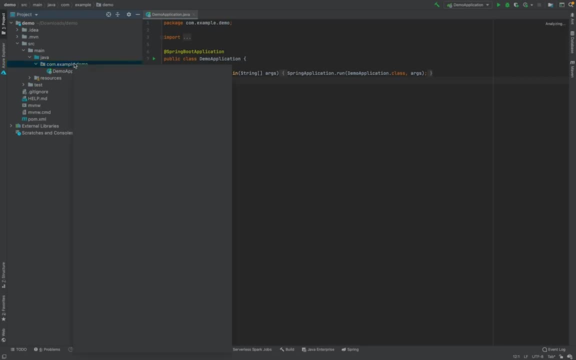 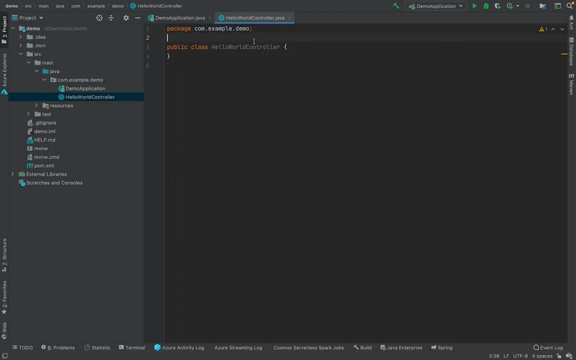 So I will just click here New Java class And I'll just call this hello world controller. So within our hello world controller class here we need to define this as a REST controller, So we'll say REST controller. And then we need our first method. that will return something where we'll add our endpoint. 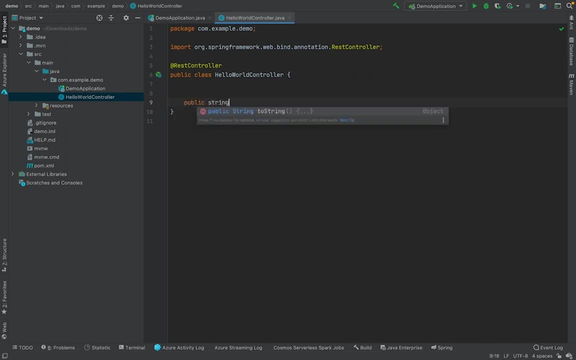 So we'll create a product method here that returns a string, And this is just to be hello world. That is to take no parameters, But it's to return the string hello world. This is my app Like such, And then we need to define the request mapping on top of this method. 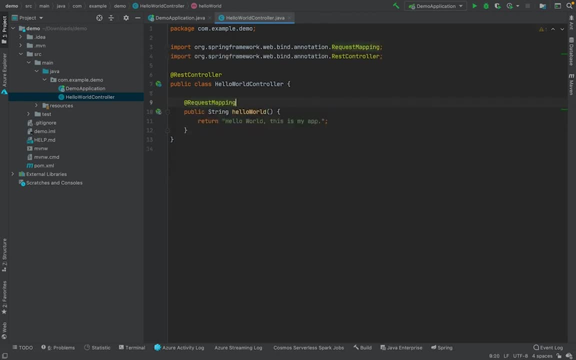 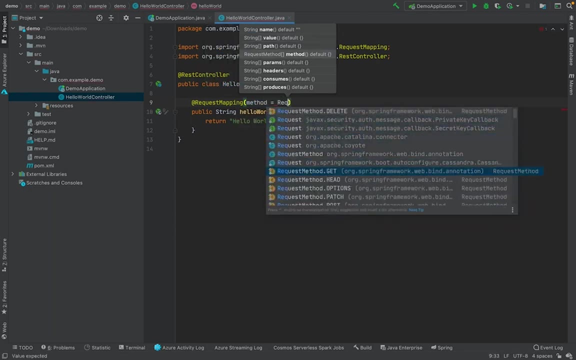 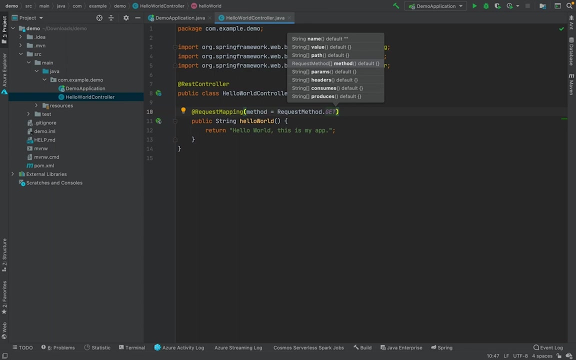 So we'll say request mapping, And here we need to say what method we want. In this case we want a request method, get, Because we'll just be returning. So within REST applications there is the get, post, put and delete, Which is the most commonly used. 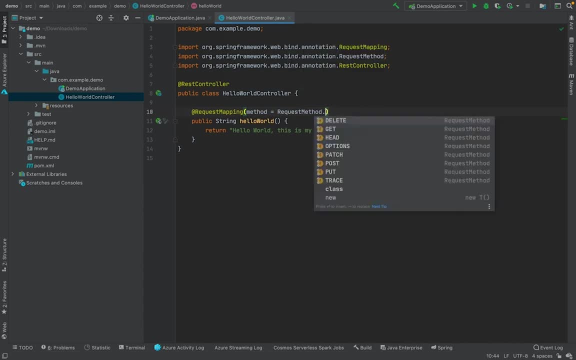 And you can use all of these here, If I just change this. There is also a few others, But the previous four is the most commonly used, But in this case we'll stick with the get. So then we need to define the path that you need to enter in order to activate this method. 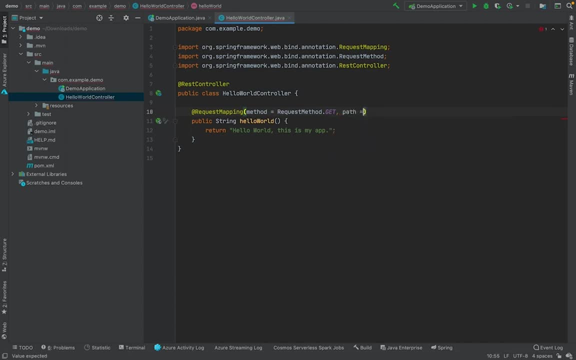 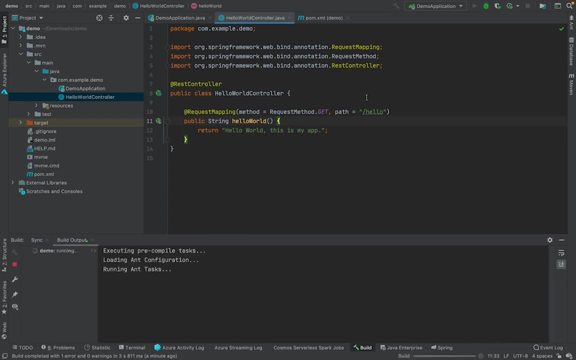 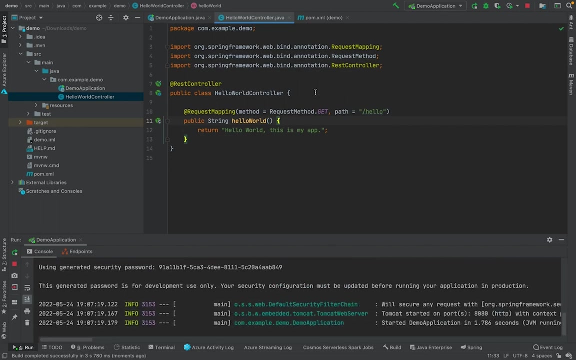 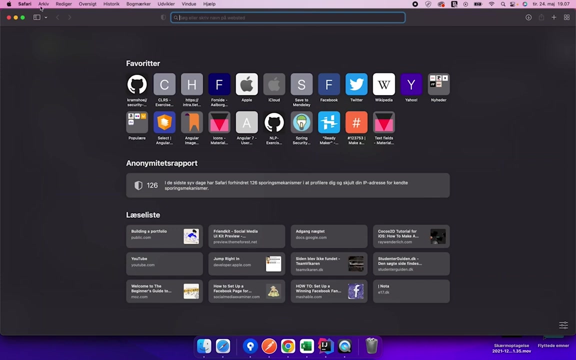 And get our string returned. So we'll say path And here we'll just say hello. So let's try to run this. So the Tomcat has now started up with our application. So let's take our browser here And say localhost. 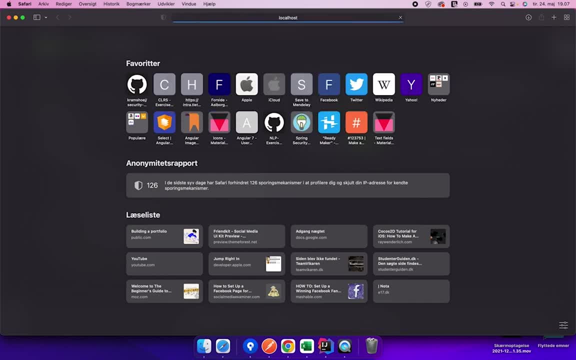 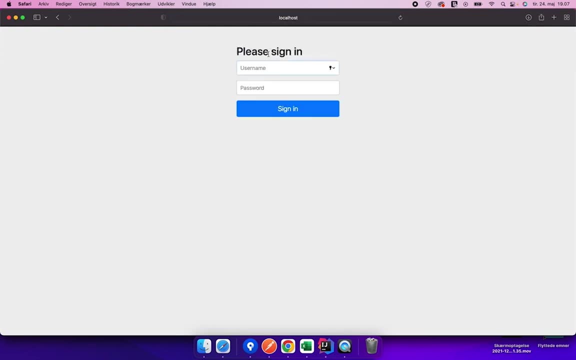 And instead of this we'll say it. And as you see, here we get to login And even if I try to say hello, It gets to the login page, And that is because we activated An added dependency spring security Which, by default, at 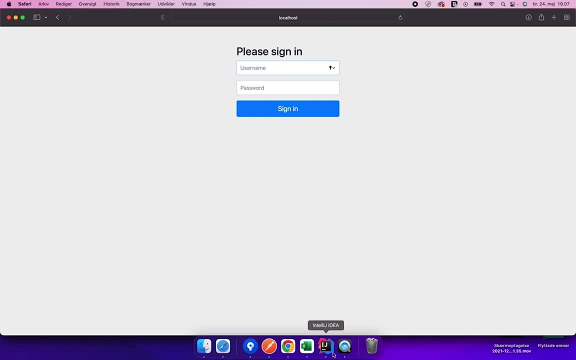 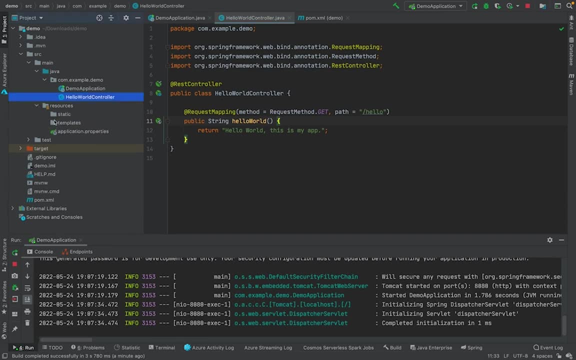 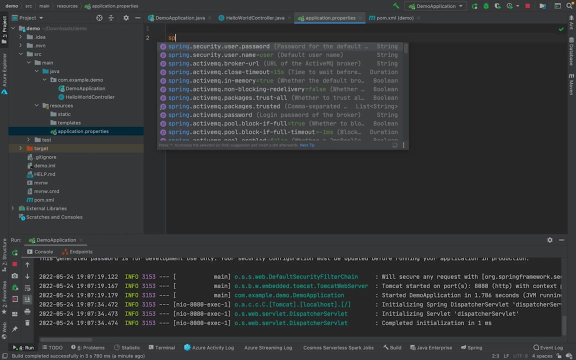 Basic authentication, meaning a user and a password. So let's go back to our application, Then we'll go into The properties file. So So we'll go in here in the application properties, Then we'll say So, we'll say spring. 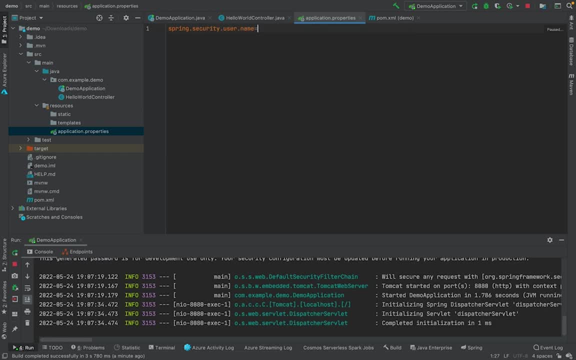 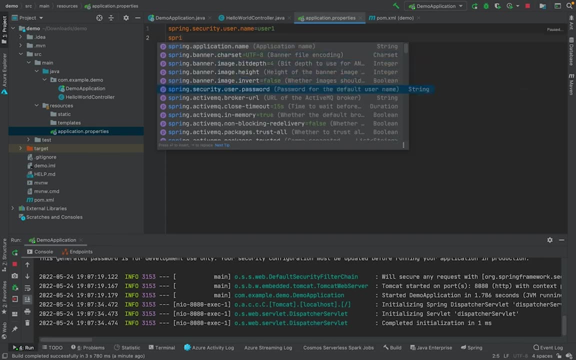 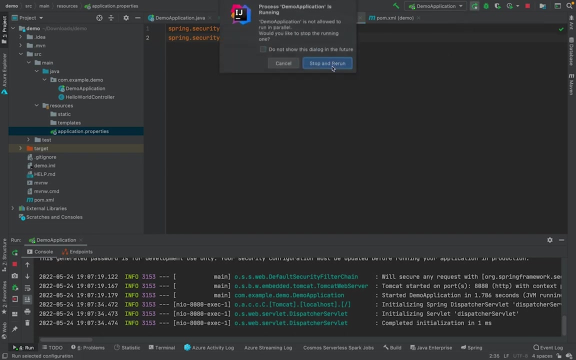 Security User name, And this is just going to be User One And we're going to say spring Security User Password And that is the password. So that will just be one, two, three, four, And this is the way that you can control. 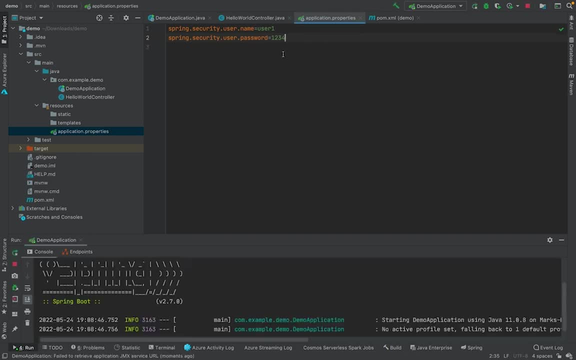 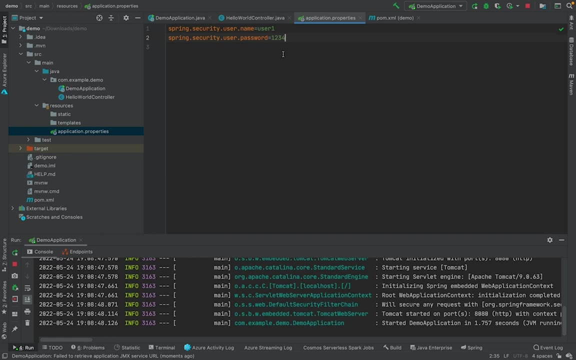 The basic authentication for a single user Just by default in spring security. Then spring security also support more advanced Security where you can have User management And you can have different users running. But that is out of scope for this video. You can, of course, add upon this. 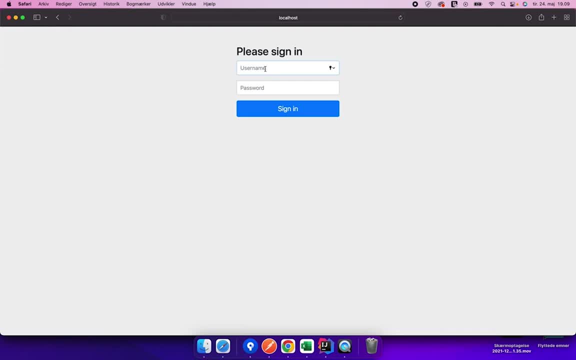 On yourself. So let's head back to our application. Then we'll say user one, Password, one, two, three, four And Use it like this: One, two, three, four. And here it said variable error, And that is because we are now not at the. 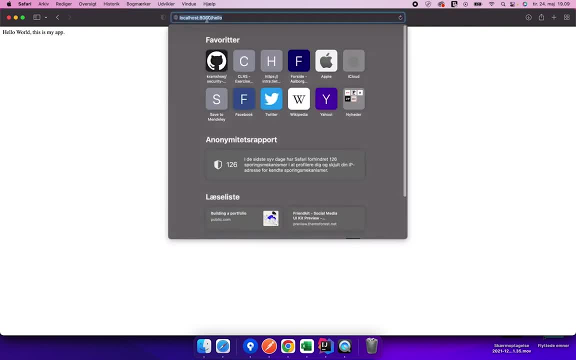 Hello. So let's try to do this. And when we insert the page On the Endpoint and port that our local host, Tomcat, was running, And then the path We defined in the code, slash, hello, We got to the hello world. 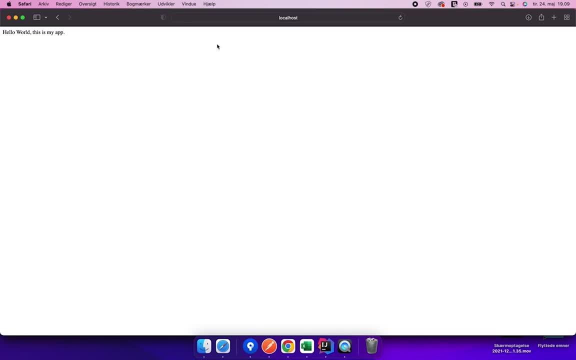 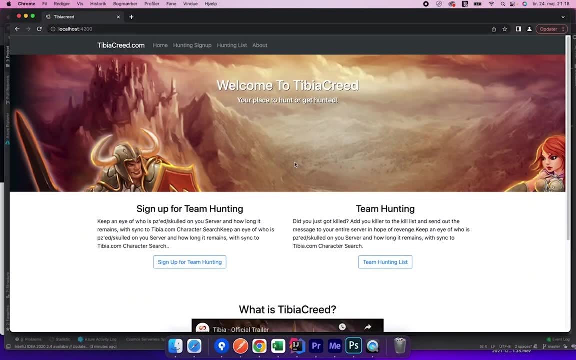 This is my app And we had basic authentication to get to this. So this is how you make a simple REST API in Java With basic authentication. This tool- we're going to look at How we do Angular- Can make a call to a backend. 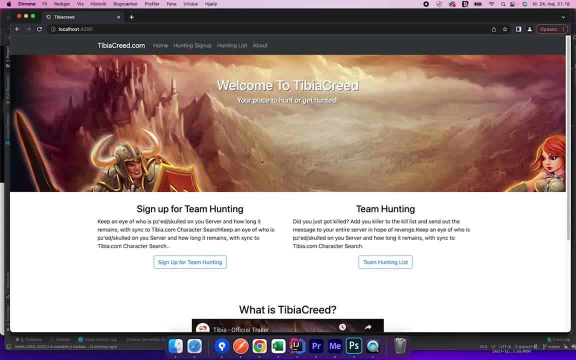 Make it return a string to us And then put it in the frontend in our Angular app. So I have this example Angular app right here. So what I wanted to do Is to, when I click this button, I wanted to Return. 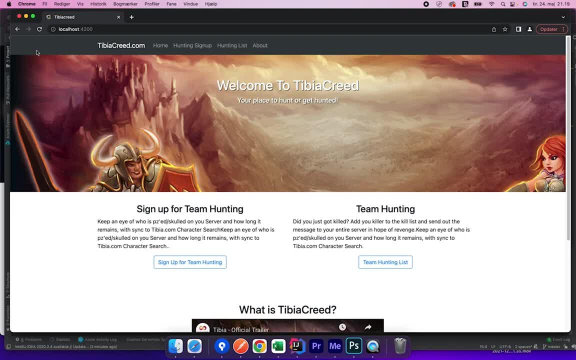 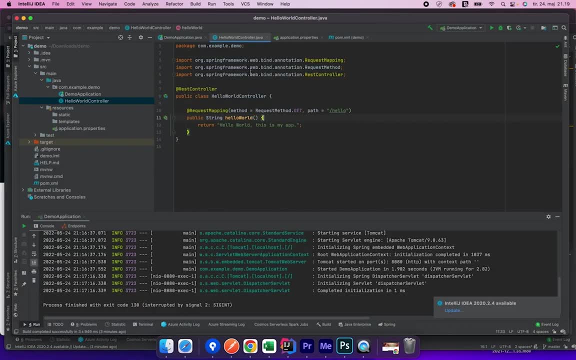 And display a string From my backend. So let's just minimize this. So here I am in the Angular project And in my backend I have this demo Hello world That I have made Using A tutorial Handwritten academy. 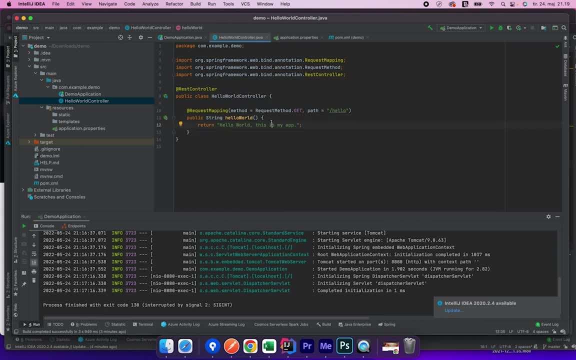 So you can look up that if you want to make it as well. But basically what this Java API do Is to, whenever you hit the endpoint, Slash hello. It will just return a string: Hello world, This is my app, So that's it. 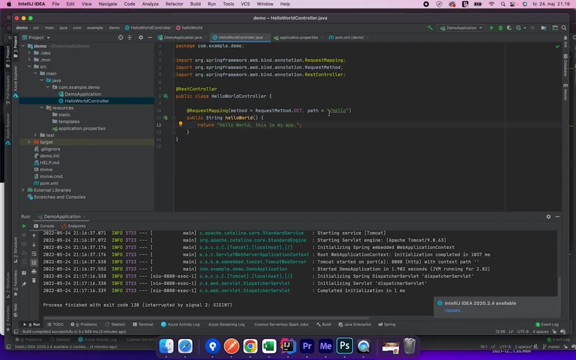 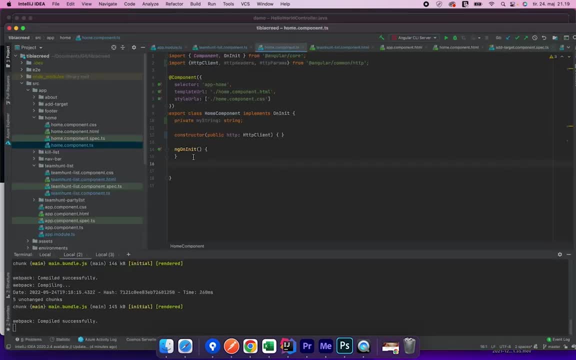 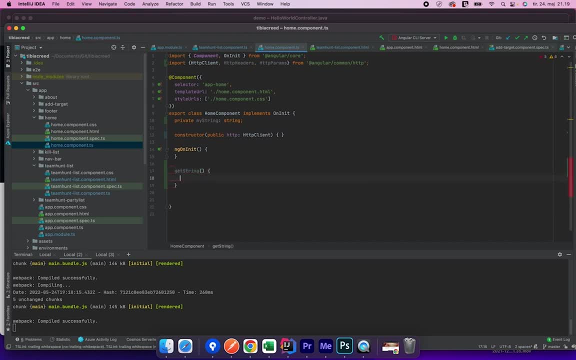 That the button should activate. So I will call this SketchString And it Takes no parameters, Because it's Just a simple get that We train this string, Apart from the method I have Made my string here, Which is where i will store. 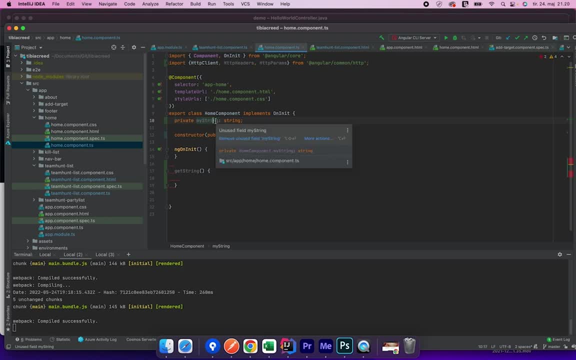 My string And also the variable that I will Make Attachments to In the front of them. So, once and then i have imported the http client from the angular common library, where i then have made this viable or variable in my constructor called http, because that is what i'm going to use. 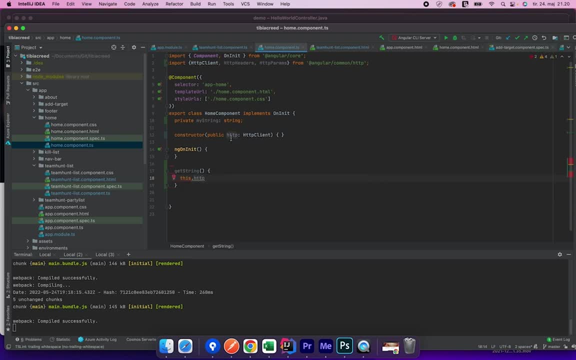 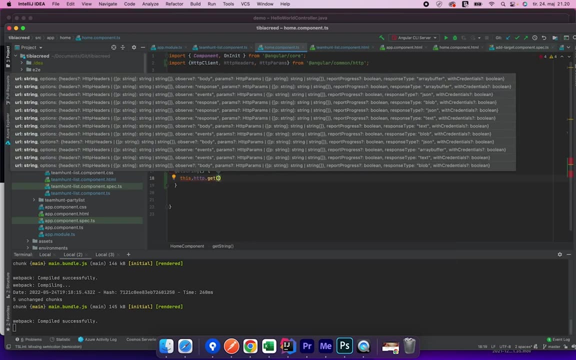 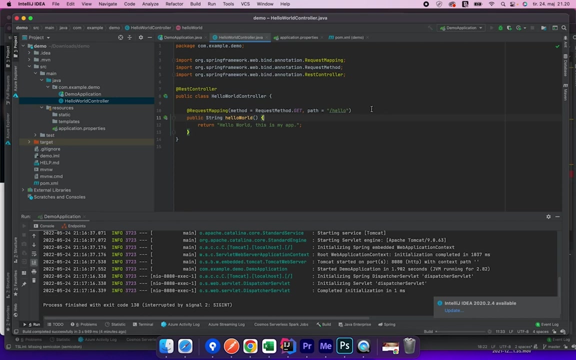 to call the back end. so i'll take this slash http or this variable here, then i will say get, because i make a get request, then i need to input the url to my backend. so let's go back here. so i will just start this up and then i will try to call it, just to make sure everything works. 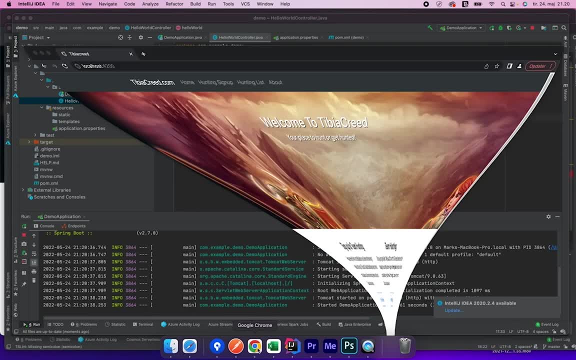 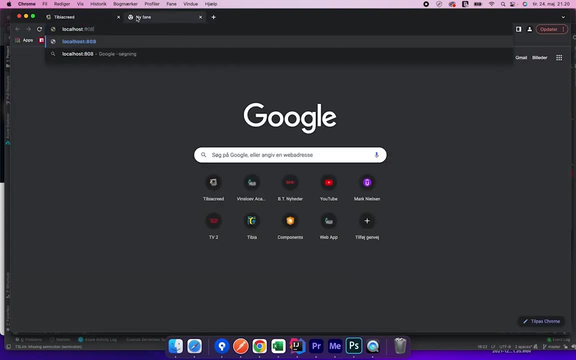 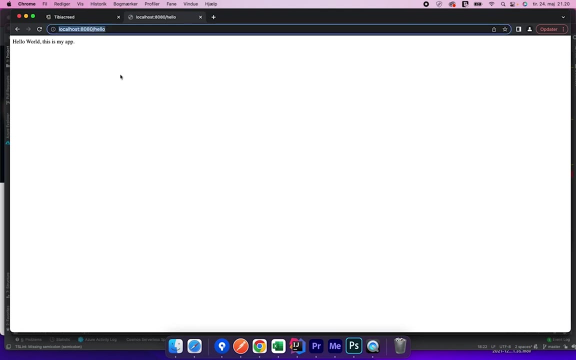 as expected. so it's already running. now i'll go back here and i will say local 88 and then slash hello. and i can now see that it's working. so i can just copy this url where i returned my string, go back into my project, then in the url i: 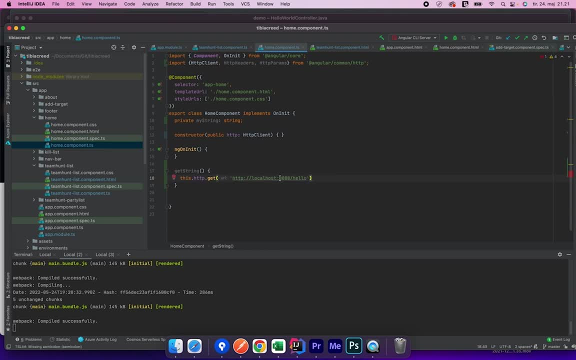 have simply put in this url here for localhost for regating slash hello, and then i will subscribe to the call that i'm making here so that i will, so that angular will be aware of when the response is returned and update my robot based on it. so i'll make a response here, type. 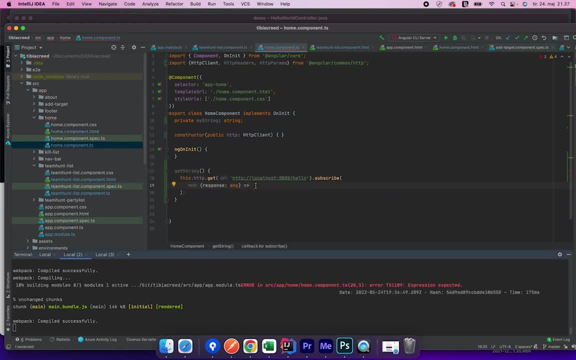 any, that could be a string. so i will say that response. this is purple here, or maybe i should call this response, and since our response object in this is coming from the back end in the verbal response you say: go into the responding verbal and then take the value from response and that we are signing to. 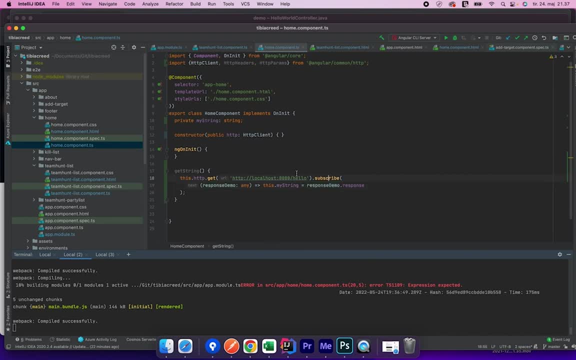 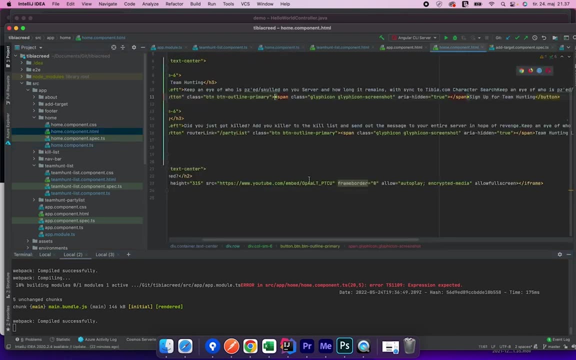 this my screen lecture, so this is what we need to make, a little method, to call it again. now we need to attach this to our front end while we have your work to do, and in here i just need the button that i want to initialize this call. 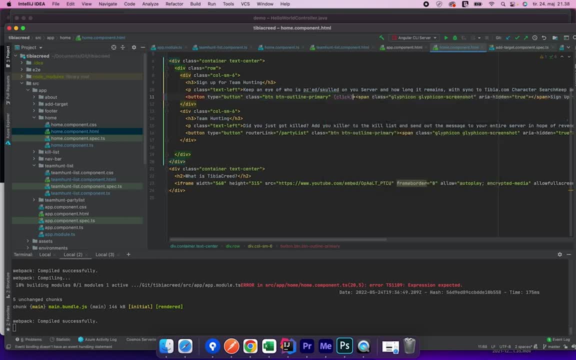 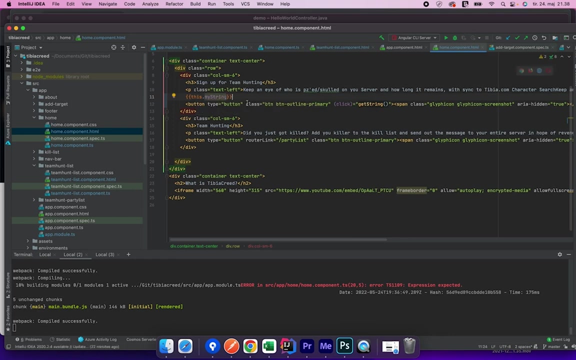 so within this button tag i can just say click, and then i can open to my get string method, and now i just need to show the value that is being saved. so this is my string. so now, whenever i click this button, it will call the method that we have created here, which will then update the variable. 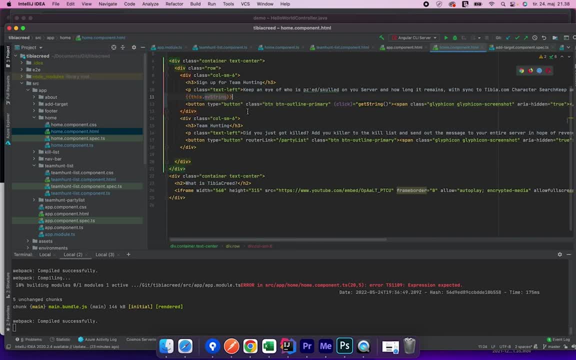 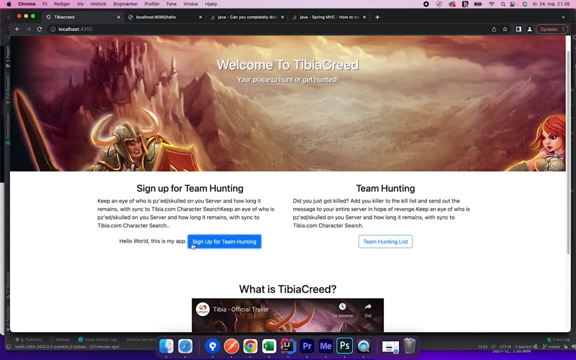 value my string, which is then displayed front end. so let's see this. so if i click this button now, as you see, hello world, this is my app. so this is how you can connect angular frontend to, for example, java backend or basically any backend that you have. 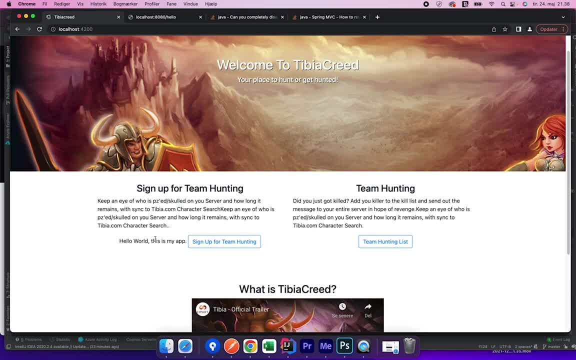 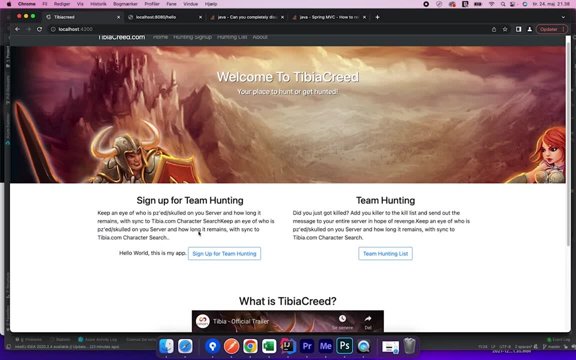 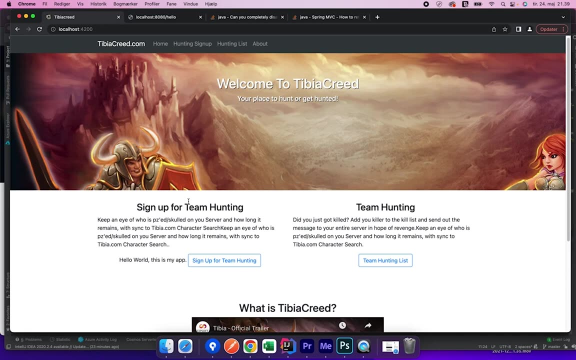 that will provide an api that you can call. in this example it just returns in the string, but you can basically make it between complex objects that you can then use to manipulate the front end. but for an example, based on pretending the user that has logged in, or if you want to show some